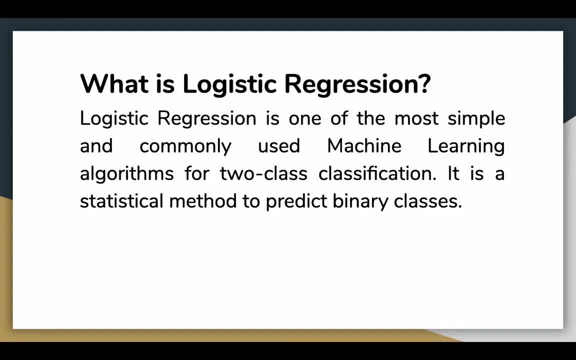 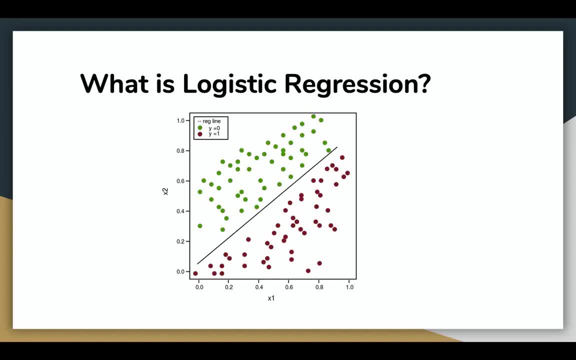 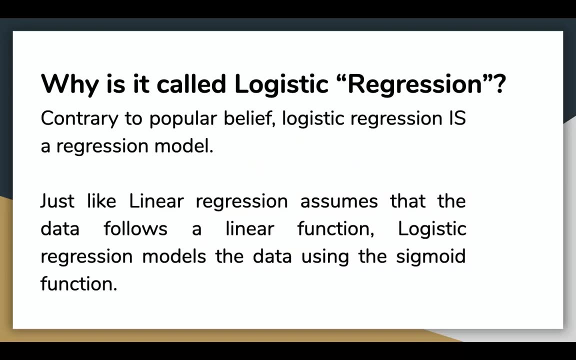 Logistic regression predicts the probability of a binary event utilizing a logic function. As we can see here, we need to categorize the data in two different categories, and our job is to define the line which does that. Now, why is it called logistic regression if it's a classification mechanism? 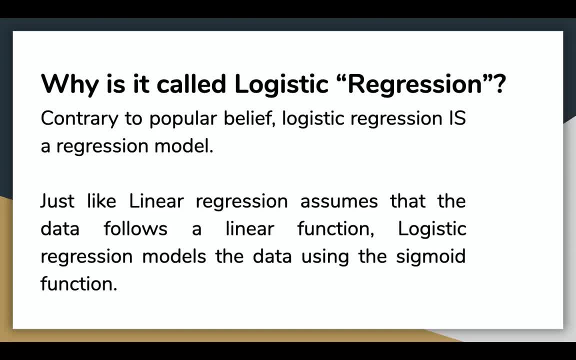 Contrary to popular belief, logistic regression is a regression model. The model builds a regression model to predict the probability that a given data entry belongs to the category numbered as 1.. Just like linear regression assumes that the data follows a linear function, logistic regression models the data using a sigmoid function. 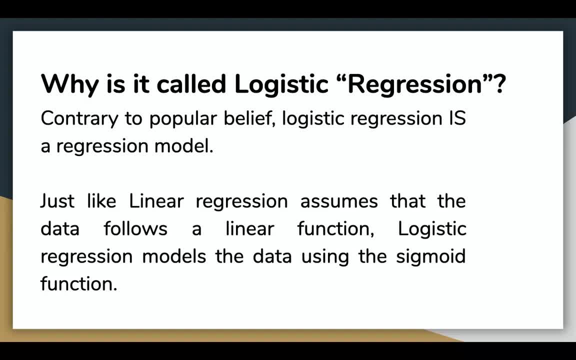 Linear regression gives you a continuous output, but logistic regression provides a constant output. An example of continuous output would be house price prediction or logistic regression. An example of discrete output is predicting whether a patient has cancer or not, or predicting whether a customer would click on an ad or not. 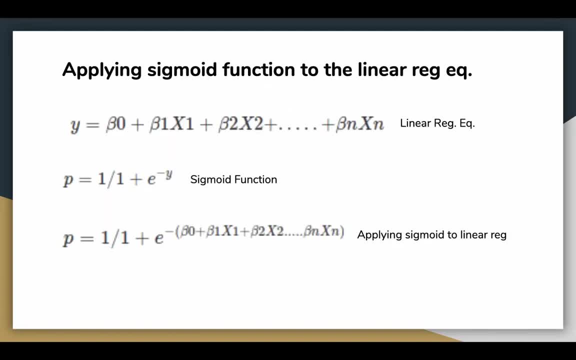 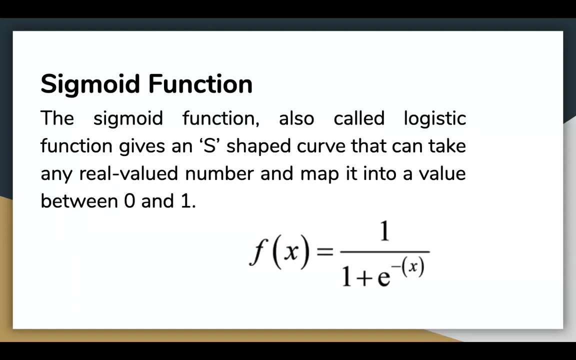 Now let's modify the linear regression equation we had seen in the previous video. for logistic regression, We apply something called as a sigmoid function on the linear regression equation. Let's see what the sigmoid function is. The sigmoid function, also called the logistic function, gives an S-shaped function. 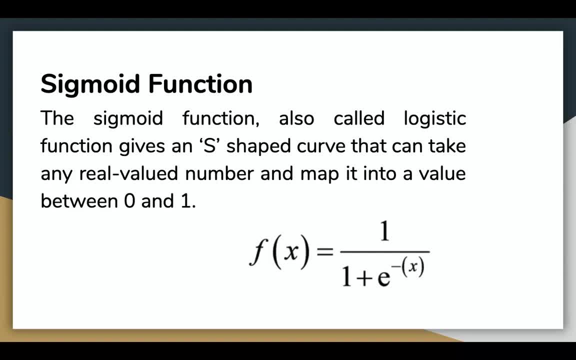 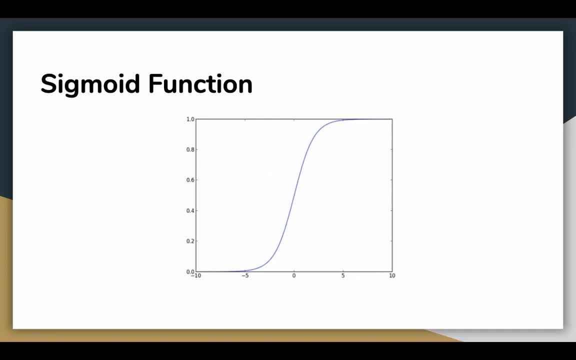 It gives an S-shaped curve that can take any real valued number and map it into a value between 0 and 1.. If the curve goes to positive, infinity y predicted will be 1 and if the curve goes to negative, infinity y predicted will become 0.. 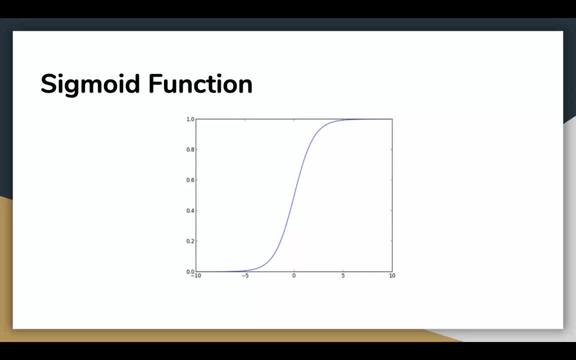 If the output of the sigmoid function is more than 0.5, we can classify the outcome as yes or a 1. And if it is less than 0.5, we can classify it as 0 or a no. For example, if the output is 0.75, we can say in terms of probability, as there is 75% chance that patient will suffer from cancer. 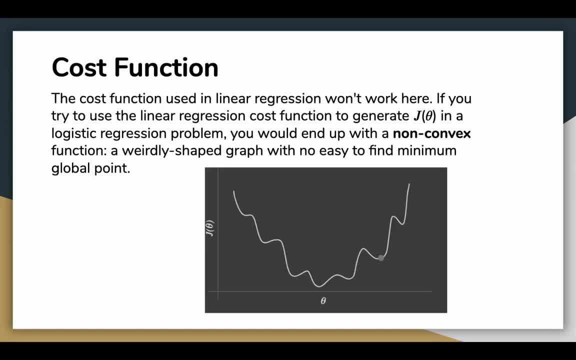 Just like we have a cost function in linear regression, we need one for logistic regression as well, which has to be reduced to obtain the best fit line. But the cost function used in linear regression will not work here If you try to use the linear regression cost function in a logistic regression problem. 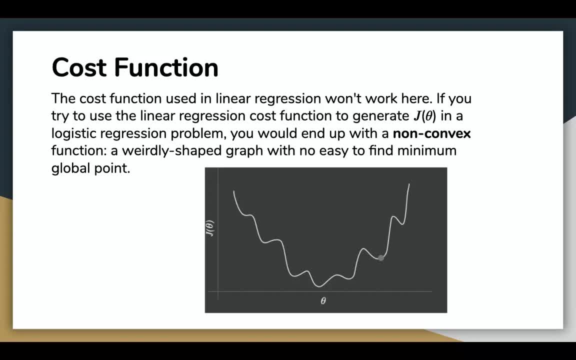 you would end up with a non-cost function. For logistic regression, the cost function is defined as a weirdly shaped graph with no easy way to find the minimum global point. Hence we have a different cost function for linear regression. For logistic regression, the cost function is defined as: 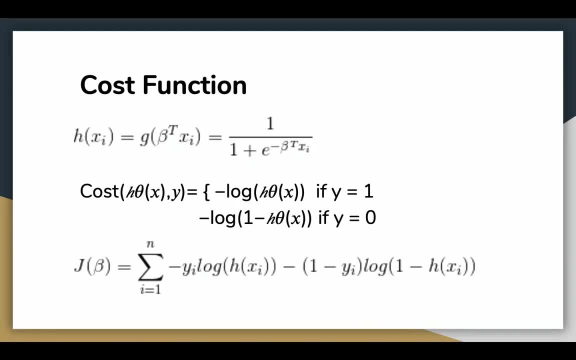 minus log h of x if y equal to 1, and minus log 1 minus h of x if y equal to 0.. This is the cost the algorithm pays if it predicts a value h theta of x, while the actual cost label turns out to be y. 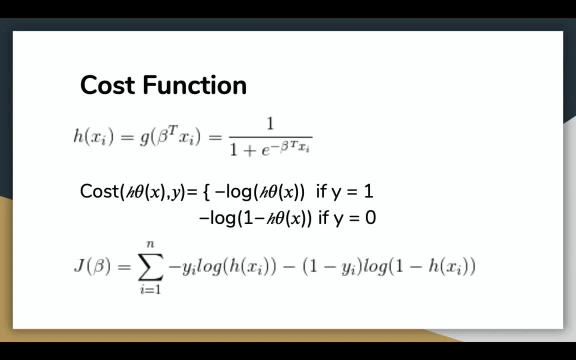 This is the cost the algorithm pays if it predicts a value h theta of x, while the actual cost label turns out to be y. By using this function, we will grant convexity to the function the gradient descent algorithm has to process. There is also a mathematical proof of how we get this cost function, which is outside the scope of this video. 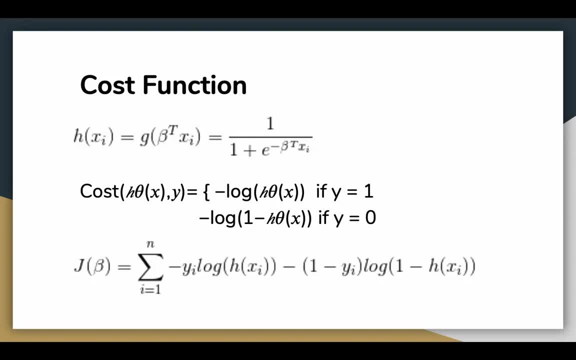 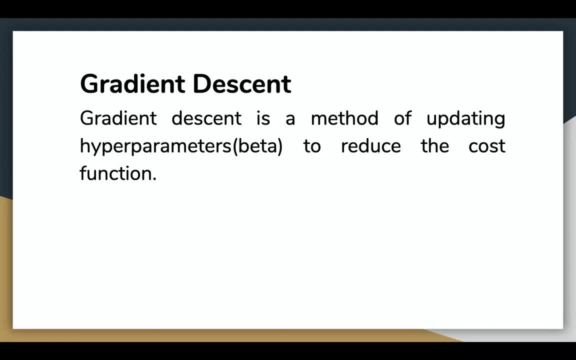 The final cost function can be seen at the bottom of the slide. Now we have the hypothesis function and the cost function, and we are almost done. It is now time to find the best values for our parameters in the cost function, or in other words, the cost function. 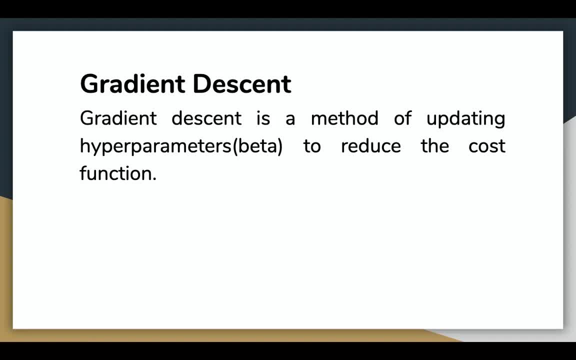 To find the best values for our parameters in the cost function, we need to run the gradient descent algorithm. The procedure is identical to what we did for linear regression. To understand more about gradient descent, please find the link in the description which will explain linear regression and also gradient descent. 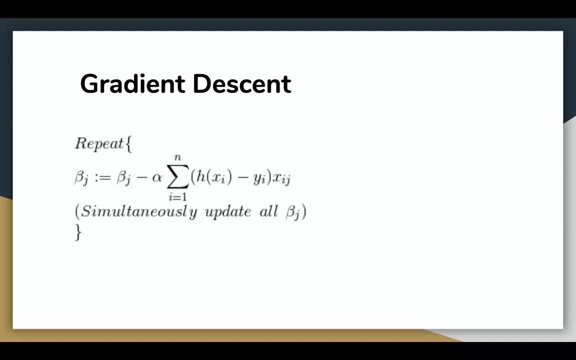 To minimize the cost function, we have to run the gradient descent function on each parameter and that is how logistic regression works. At the end we get the best parameters that can work with the hypothesis function to predict whether a data point belongs to one class or the other. 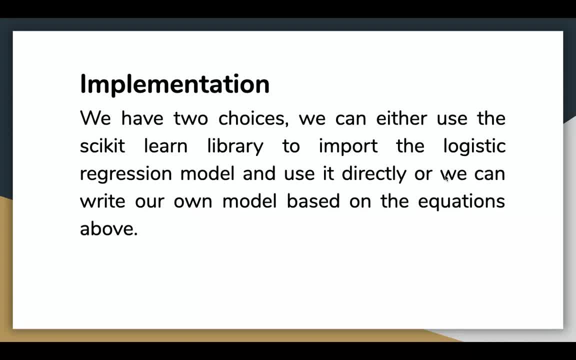 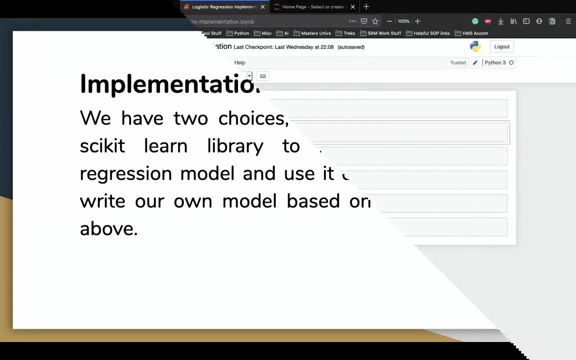 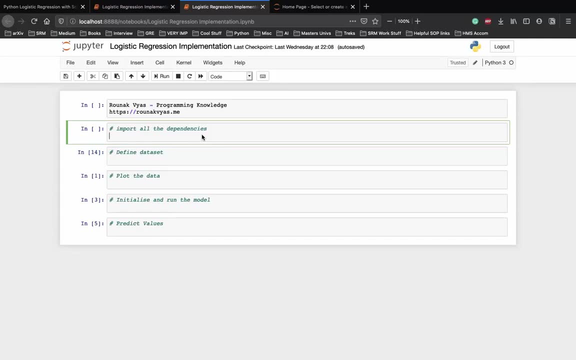 Now for the implementation. we can either use the scikit-learn library to import the logistic regression model and use it directly, or we can also write our own model based on the equations above. We will talk about implementing logistic regression. Logistic regression is amongst the most commonly known core machine learning algorithm out there, with its cousin, linear regression. 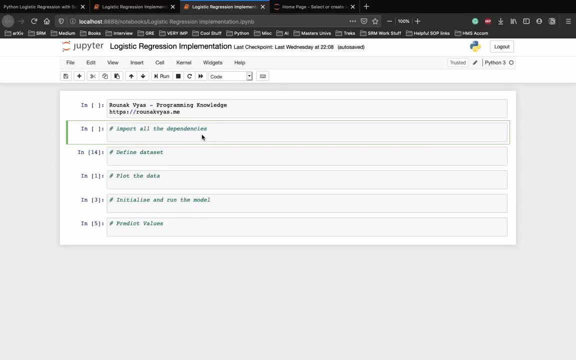 It has many applications in businesses, One of which is the pricing optimization. In this video we will learn how to code logistic regression in Python using the scikit-learn library to solve a bit pricing problem. Let's have some recap. Logistic regression is a predictive linear model that aims to explain the relationship between a dependent binary variable and one or more independent variables. 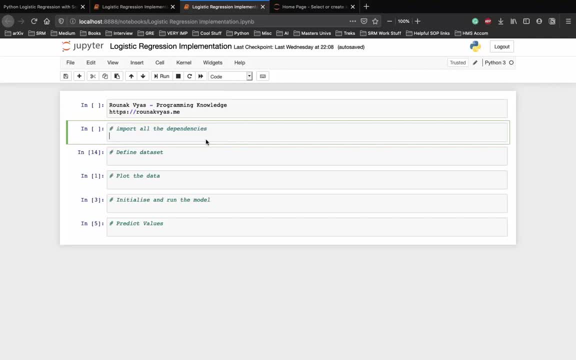 The output of logistic regression is a number between 0 and 1, which you can think of as being the probability: The probability that a given class is true or not. The output is between 0 and 1 because the output is transformed by a function, which is usually the sigmoid function. 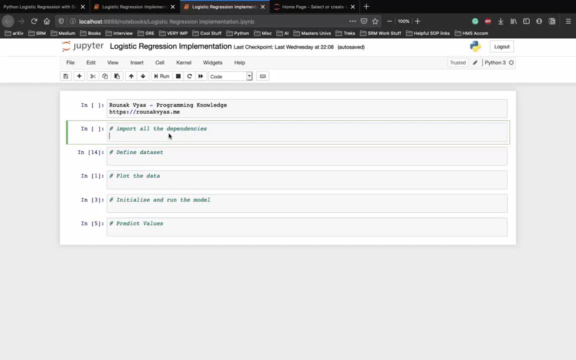 Let's start implementing logistic regression in Python with a very simple example. Note that the intent of this video is only to implement a very basic logistic regression model using scikit-learn, without using a train-trest split on the dataset and with minimum data visualization. 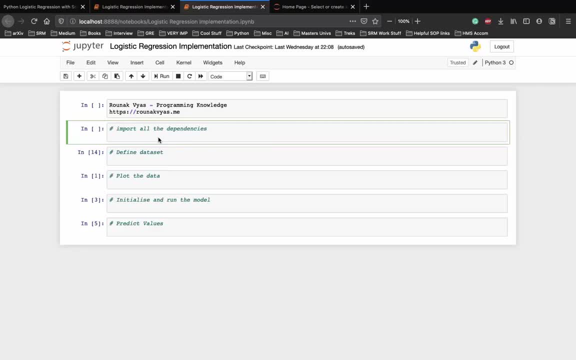 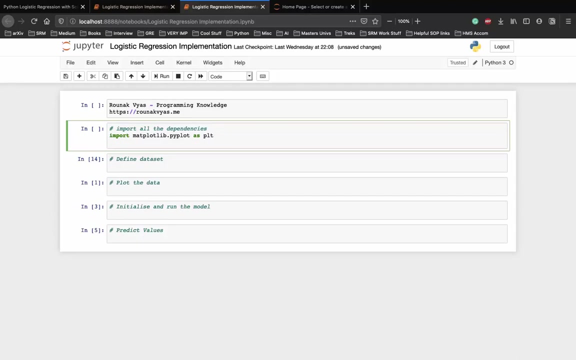 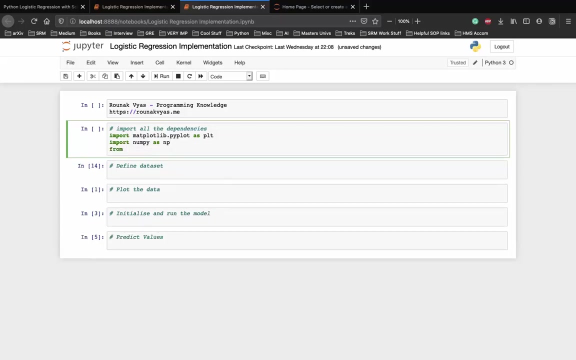 So let's start. First, we import all the dependencies that are required. We need matplotlib for visualization, So we need the pyplot as plt, Next is numpy to store our data, And finally we need the sklearn. And finally we need the logistic regression model, which we can use to filter data. 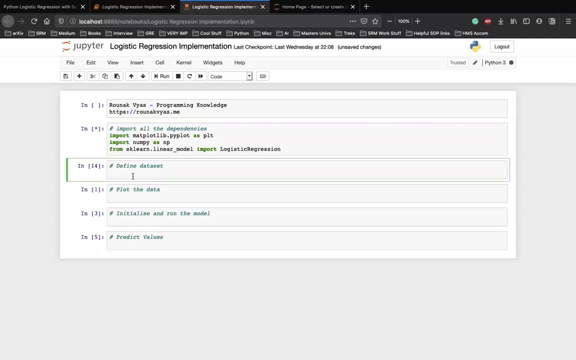 So the next is that we have to define a dataset. Let's generate a dataset that we will be using to learn how to apply logistic regression to a pricing problem. The bid price is contained in our x variable, While the result- a binary loss or one category- is encoded as 1 or 0 in our y variable. 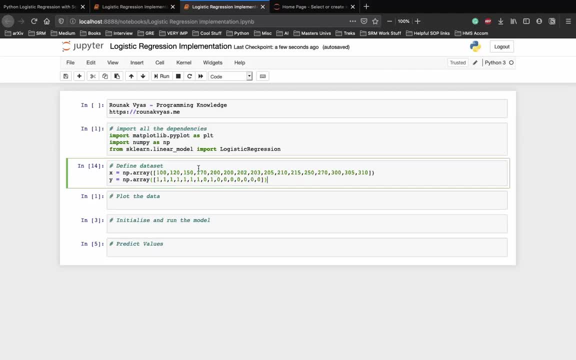 Here I have defined my own dataset, But for complicated or more advanced examples, you can also import a dataset from Kaggle and use that. Let's go ahead and visualize this data using matplotlib to gain a better understanding of what we're dealing with. 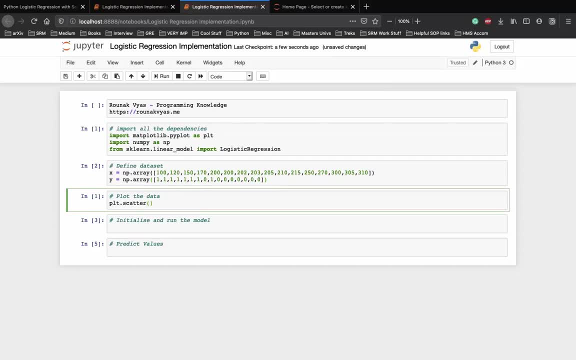 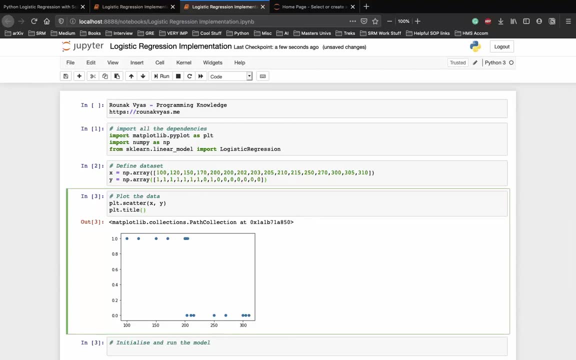 Let's have a scatterplot. Let's have a scatterplot of x and y And let's actually give it a title of pricing, bids, And the x label is going to be price And the y label is the binary output: 1 or loss. 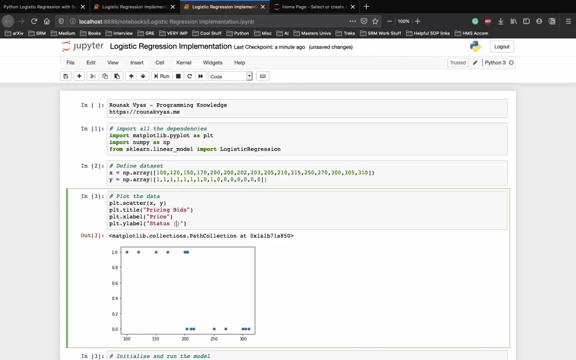 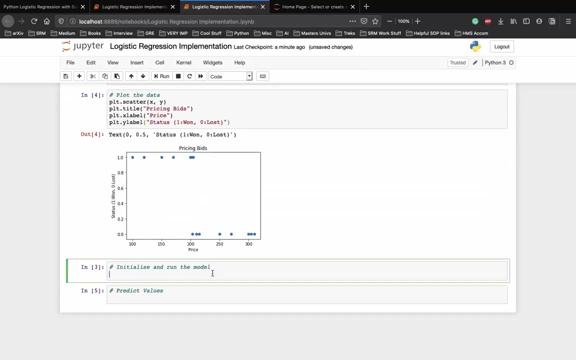 So status: 0 is a 1. And 0 is a loss. So here, each point above represents a bid that we participated in. On the x axis you can see the price that was offered And on the y axis you see the result- if we won the bid or not. 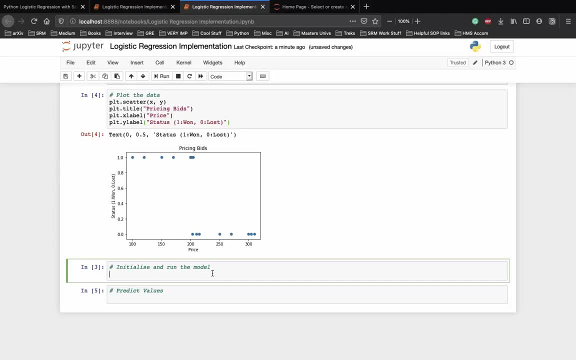 Our goal is to use logistic regression to come up with a model that generates the probability of winning Or losing a bid at a particular price. In Python, logistic regression is made simple thanks to the scikit-learn module. For the task at hand, we'll be using the logistic regression class by the sklearn linear model. 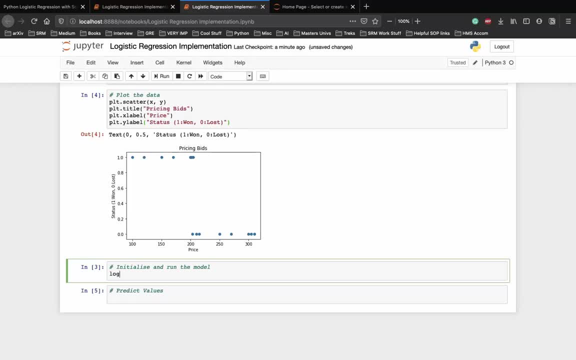 So logreg, Let that be the name of the variable And logistic regression class Where the regularization strength c is equal to 1.0.. And the solver, let that be lbfgs, which is an optimization, just like gradient descent. 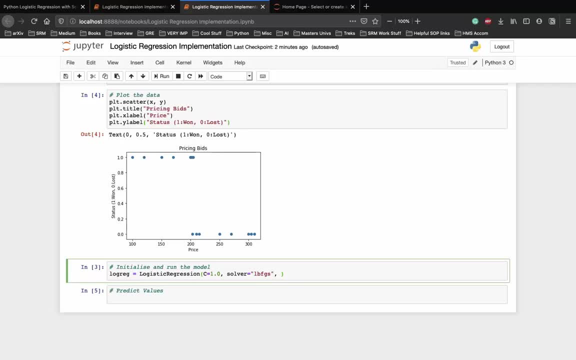 And for multiclass we specify ovr because we're using a binary classification problem here. So multiclass is equal to ovr For binary classification. The next step is to fit the logistic regression model by running the fit function of our class. 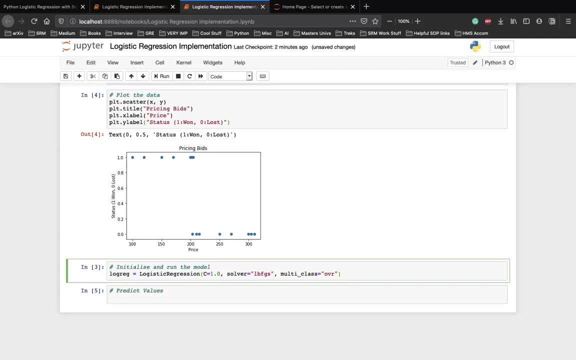 And before we do that, we transform our x array into a 2D array, as is required by the sklearn model. This is because we only have one feature, which is the price, And if we had more than one feature, our array would already be 2D.